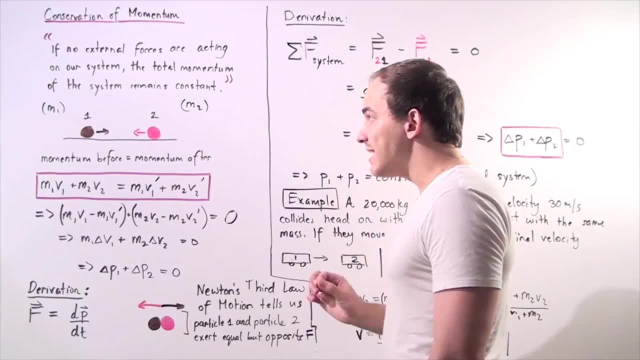 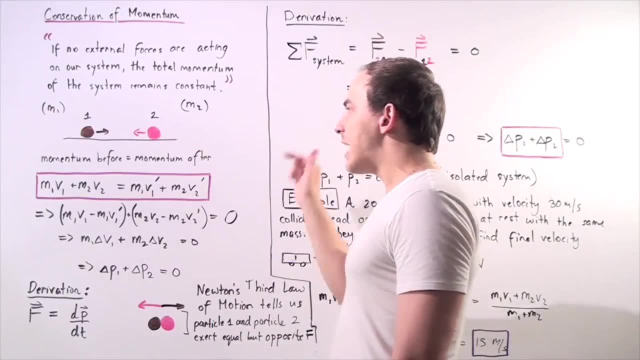 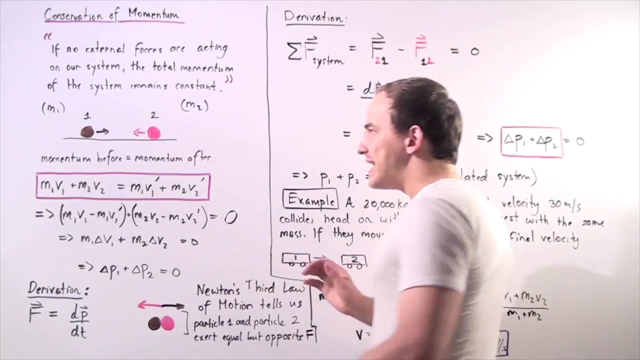 along the x-axis and its initial velocity is v1.. Now, at the same time, a second particle with mass m2 is traveling in the negative direction along the x-axis with initial velocity v2.. Now, eventually, these two particles will collide and they will bounce. 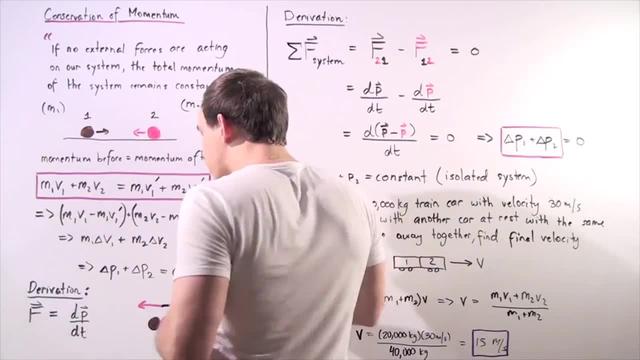 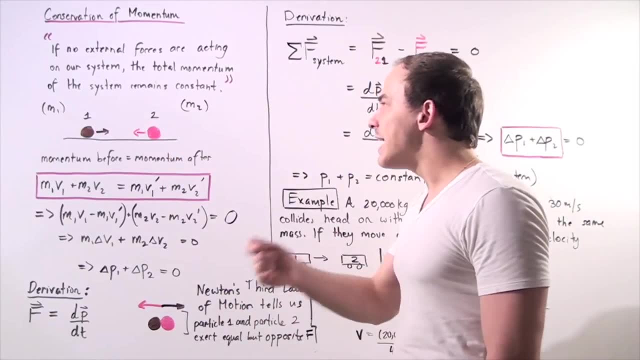 back and travel in opposite directions. So the final velocity of object one with mass m1 is v1, prime, and the final velocity after collision of object to our particle, two with mass m1, is v2, and this velocity is resumeます mvs, which is the burgeoning seam. Thanks again. 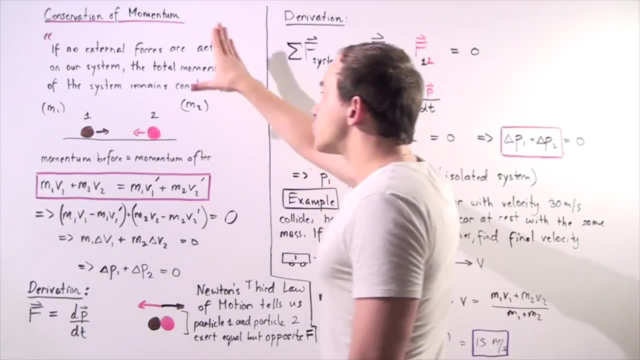 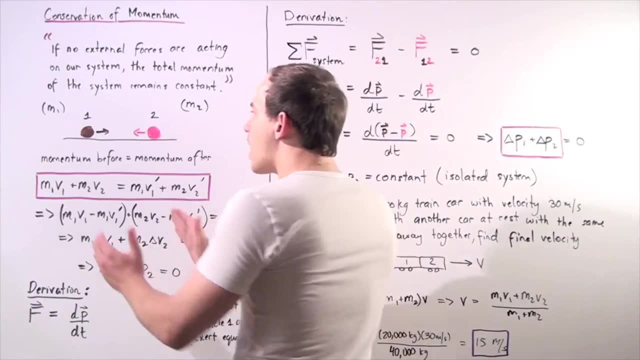 for watching and thanks for elating this video. If you have questions, you can leave them and input them in the comments. m2 is v2 prime. Now, what this law of conservation of momentum states is the following: If we sum up the momentum of our object before collision, that sum will be exactly identical to the sum of the. 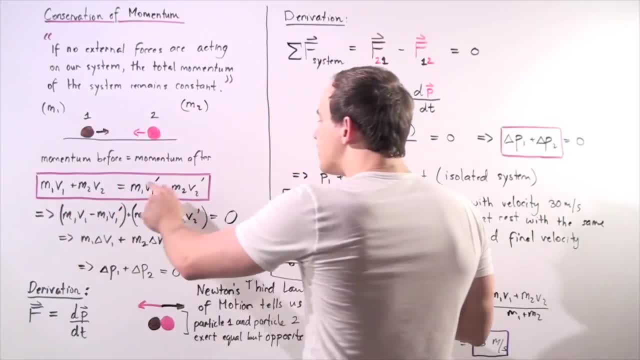 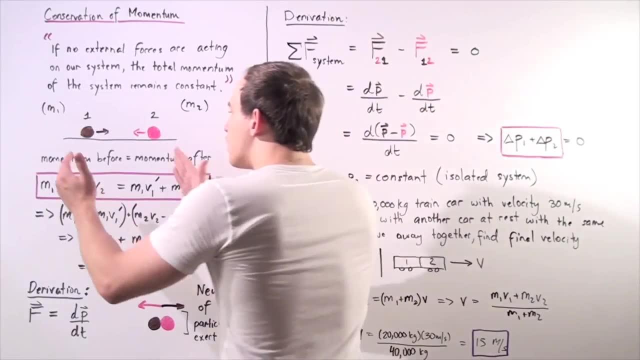 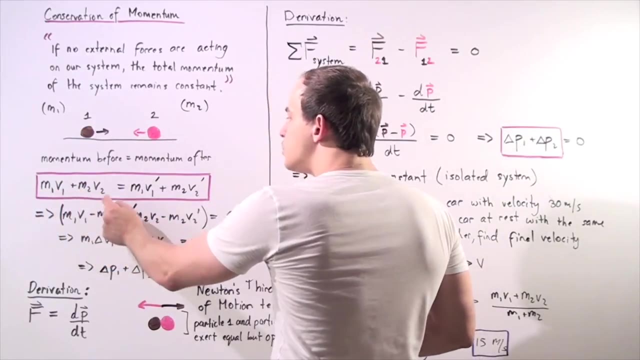 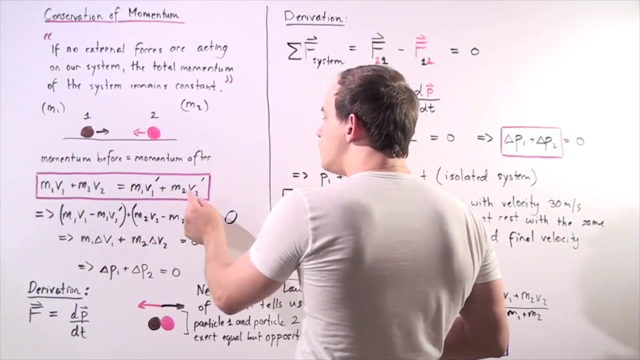 momentum after the collision And that's given by the following formula: Recall that momentum is simply mass times velocity of the object. So the momentum before the sum is equal to m1 times v1 plus m2 times v2. equals the momentum or the sum of the momentum after m1 v1 prime plus m2 v2 prime. 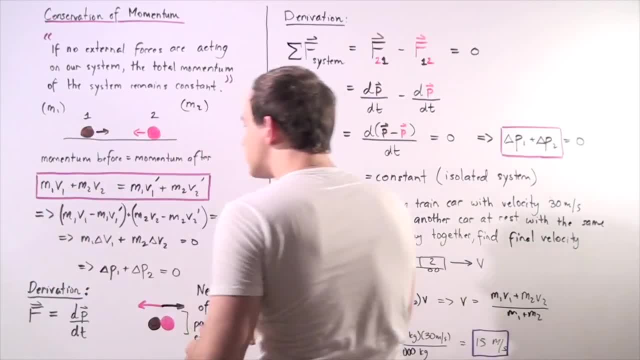 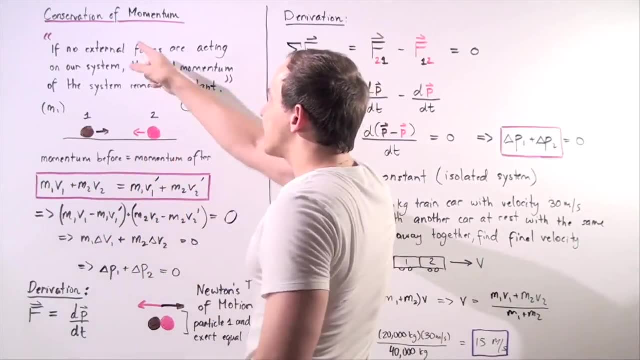 Now notice: this sum is equal to a constant. this sum is equal to a constant, and those two constants are exactly identical. And that's exactly the same thing. And that's exactly the same thing, And that's exactly what the law states, that our total momentum of the system of objects. 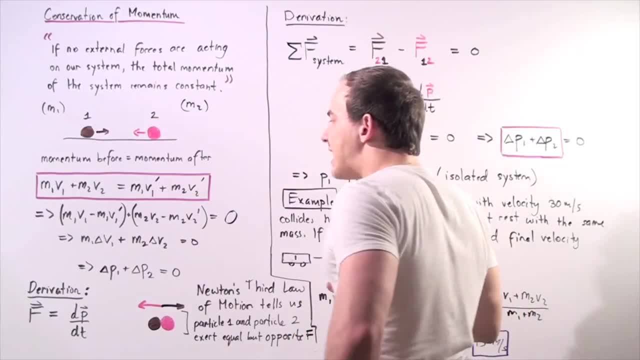 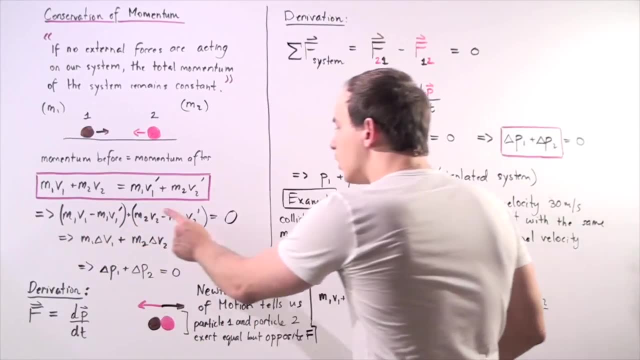 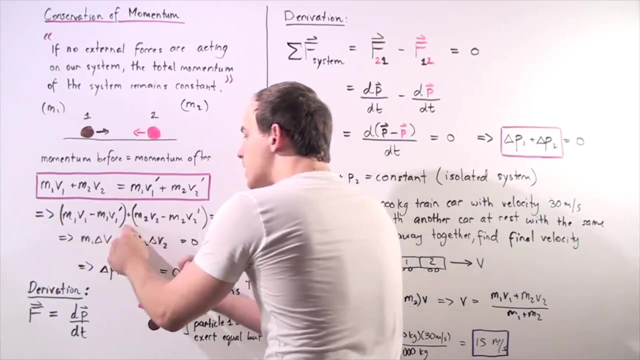 these two particles remains constant. Now notice, I can take these two terms and bring them both to the left side and we get the following equation. So this basically states that the change of momentum of object 1 plus the change in momentum of object 2 is equal to 0. And that's. 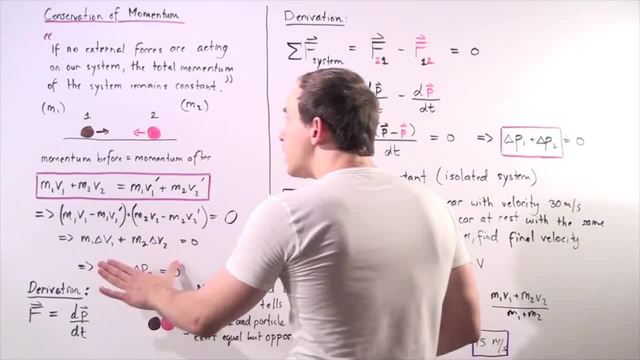 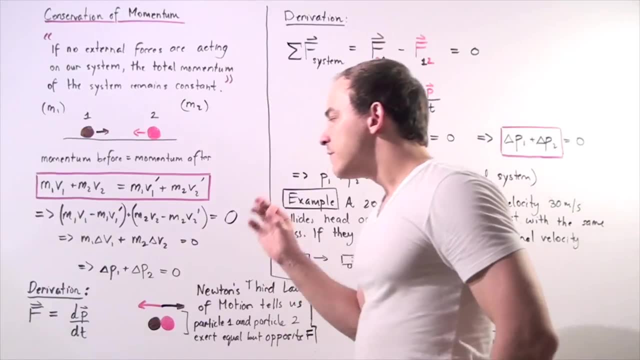 exactly what the law says, And that's exactly what the law states, And that's exactly what what we have in this equation. So this is the law of conservation of momentum. Now let's try to derive this law from Newton's second law of motion. Recall that, Newton's second law of motion. 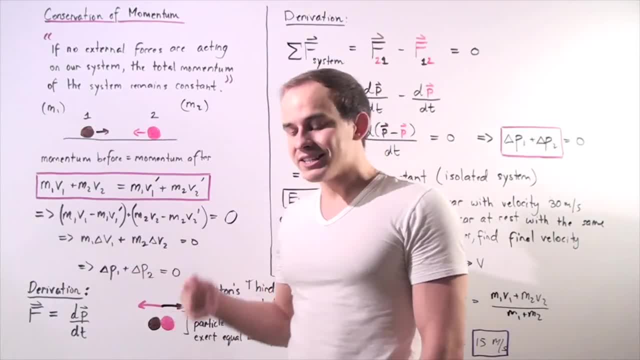 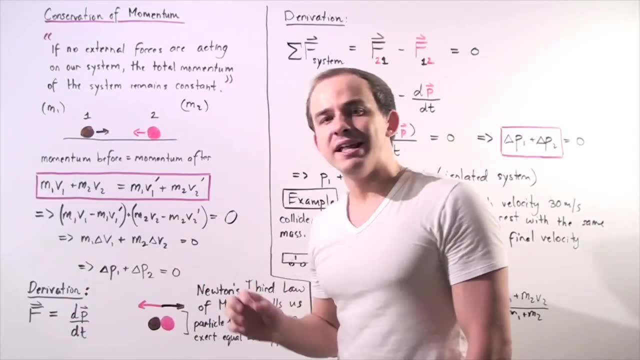 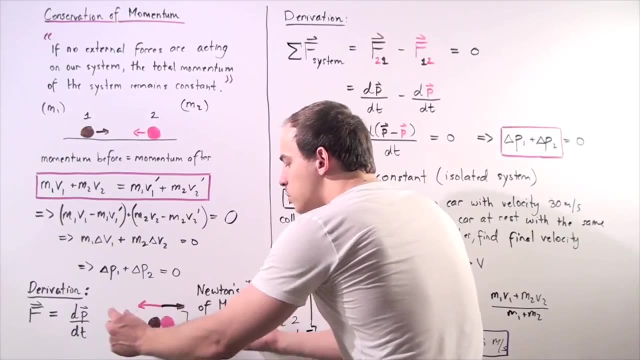 is force, or the net force acting on the object is equal to mass times, acceleration, which is equal to the derivative of our momentum function with respect to time. Now let's examine what actually takes place when our two particles collide. Well, Newton's third law of motion tells us. 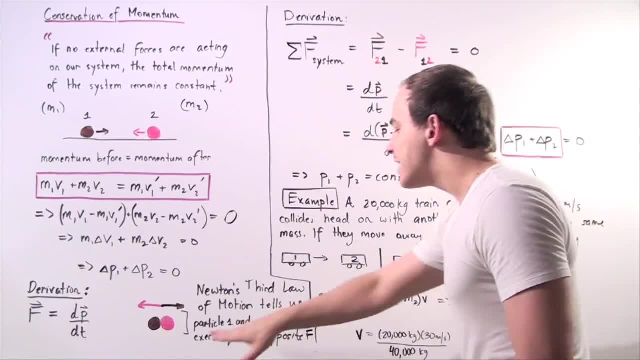 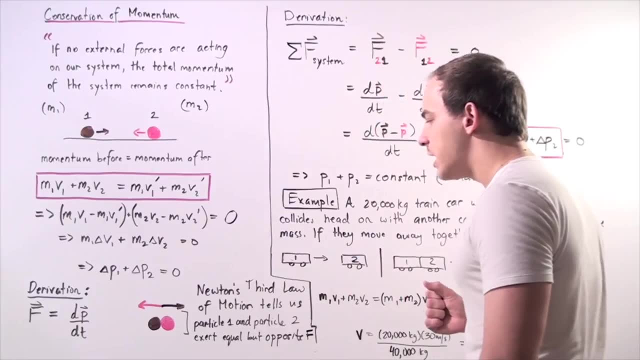 that particle one and particle two exert equal but opposite forces on one another. So this is Newton's third law of motion. So we can use this fact and Newton's second law of motion to derive the derivative of our momentum function with respect to time. Now let's examine what. 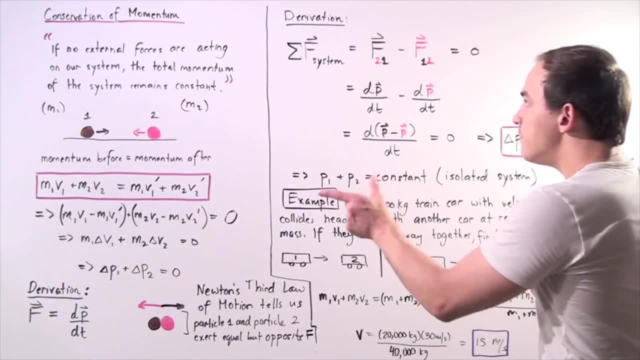 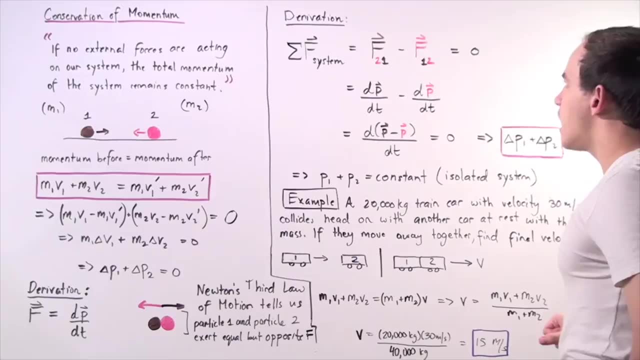 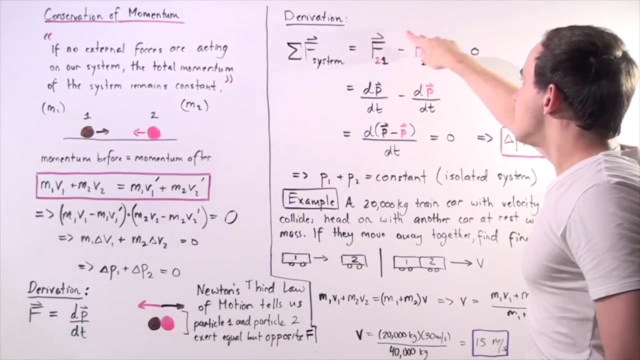 we can do to derive this equation. So if we sum up all the forces acting on our system of two objects, we get the following sum: The force created or the force exerted on object two by object one, minus the force exerted on object one by object two is equal to zero. So because this 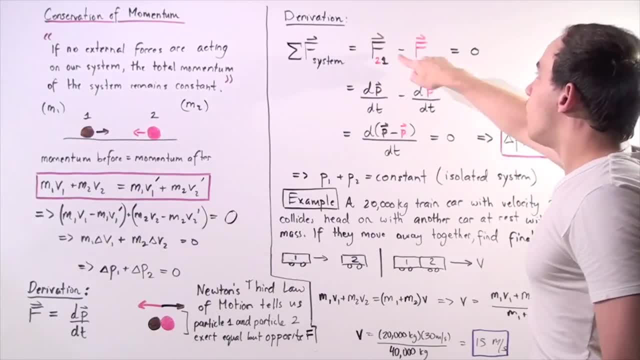 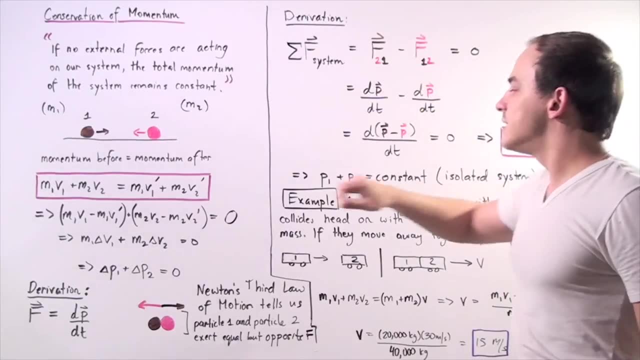 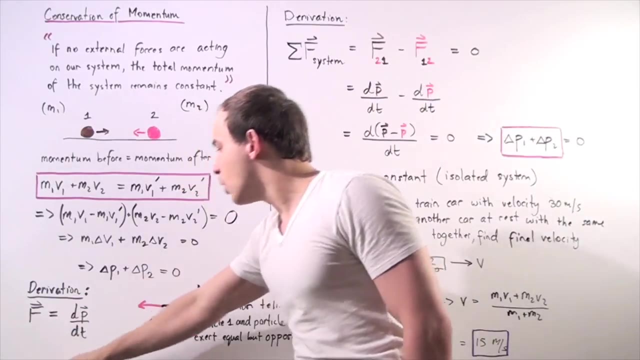 force has the same magnitude as this force, it points in opposite directions because of Newton's third law of motion. if I sum up these two forces, since they point along the same axis, the sum will equal to zero. Now, by using Newton's second law of motion, we can rewrite each. 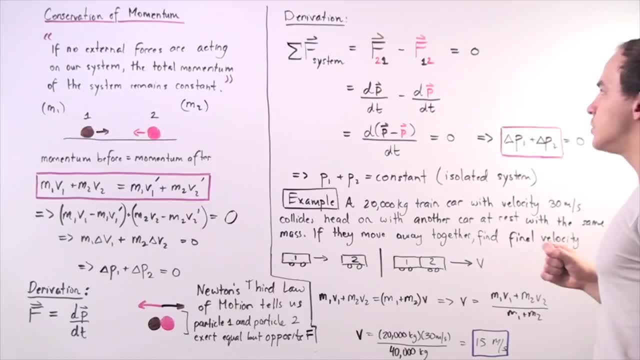 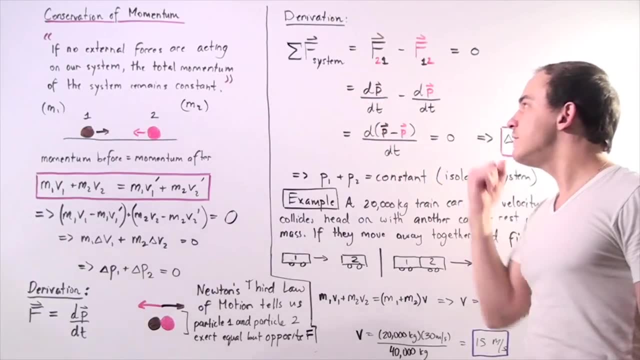 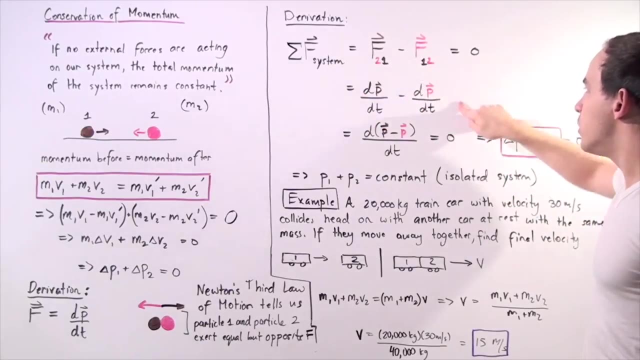 of these forces using the following representation: So the force created by object one on object two is written as our derivative of our momentum of object one with respect to time. So if we sum up the photos up here, this one is in relation to our reason: moment, force and momentum. 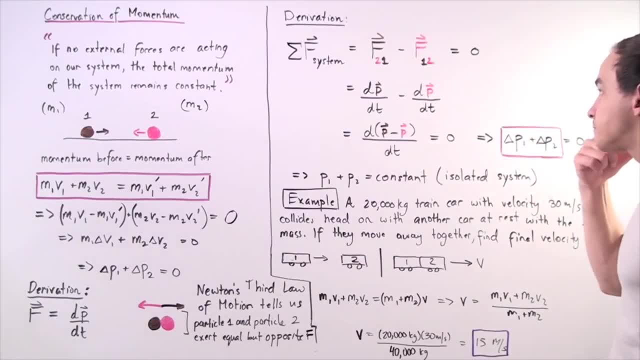 and the same folks there. one, obviously by the current器 with respect to time, done with this derivative of our objects to momentum with respect to time. So I can combine them in the following way and notice I have momentum one minus momentum two, or change the momentum one minus change in. 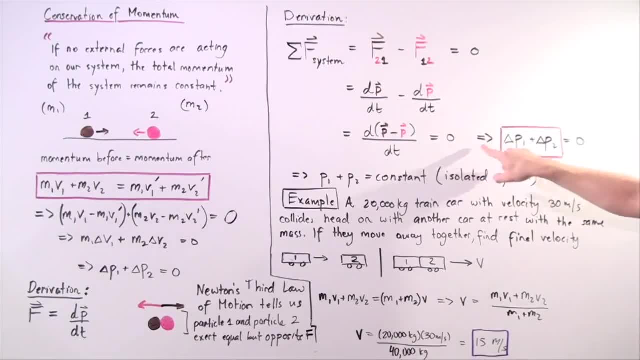 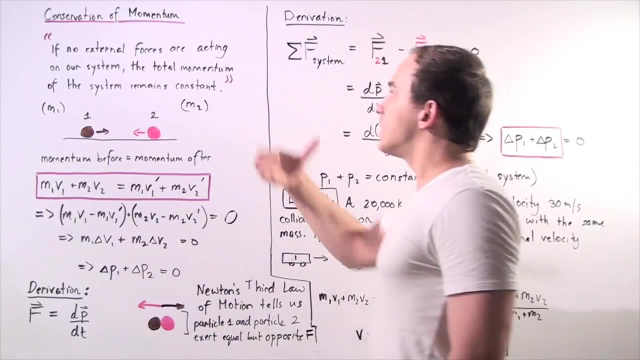 momentum two, And that equals zero, And that's exactly what we have. so this implies that this object 1 plus the change in momentum of object 2 is equal to 0, and that's exactly identical to this equation. So once again, we derived the conservation of momentum law using Newton's. 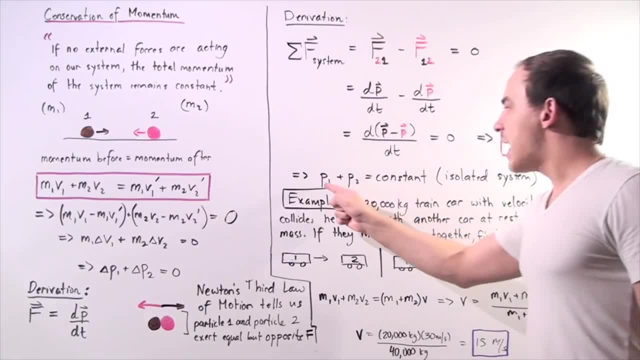 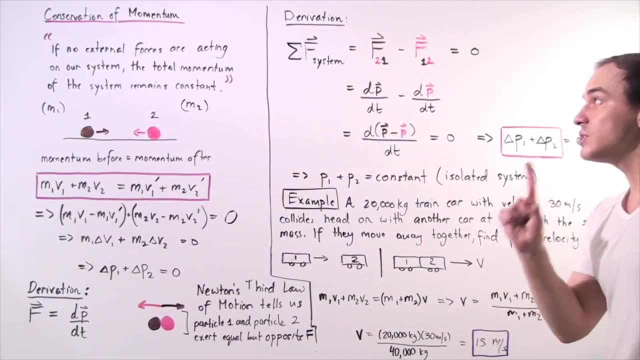 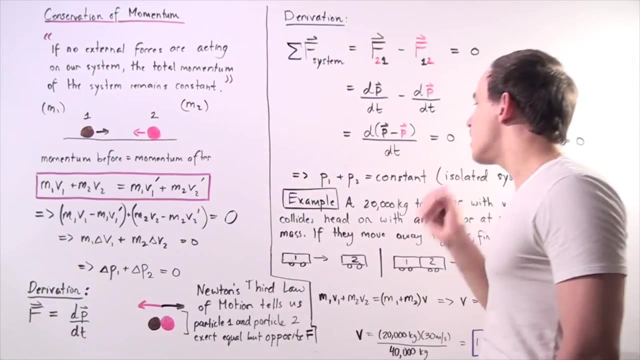 second law of motion. Now this implies that our P1 momentum of object 1 plus momentum of object 2 is equal to a constant, as long as we have an isolated system in which we have no external forces acting on our objects. So let's look at one application. Let's look at the following. 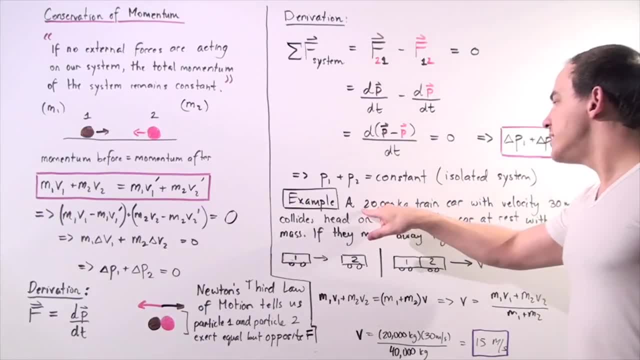 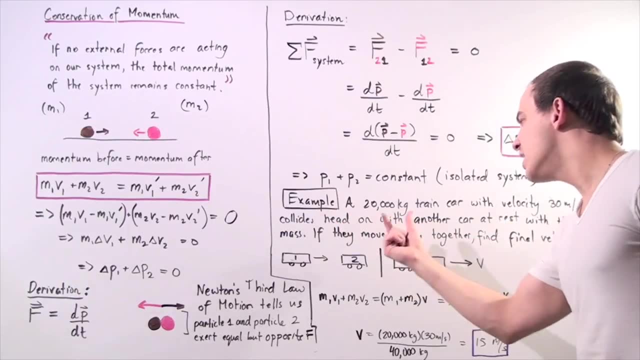 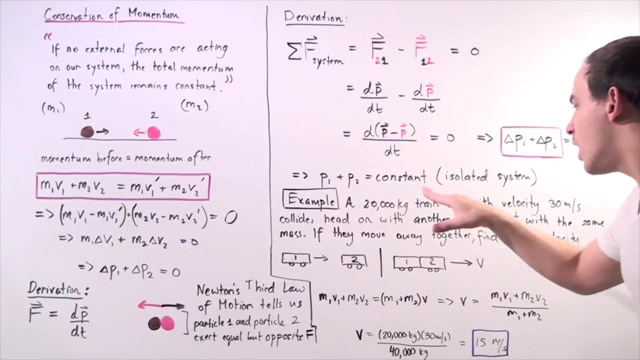 example, Let's suppose a 20,000 kilogram train with velocity 30 meters per second collides head-on with another car at rest with the same exact mass. Now if they move away together, find the final velocity. So I have: object 2 is stationary. 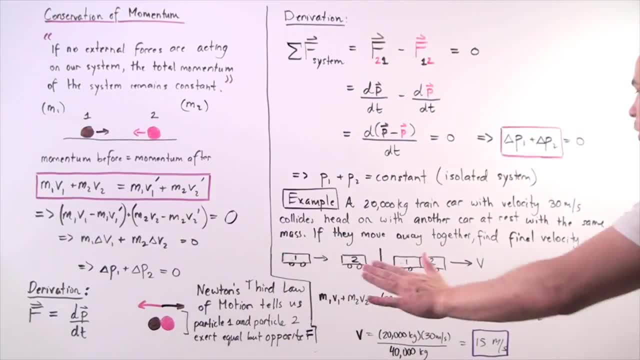 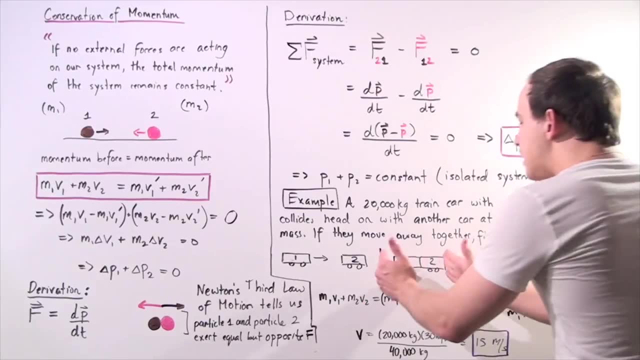 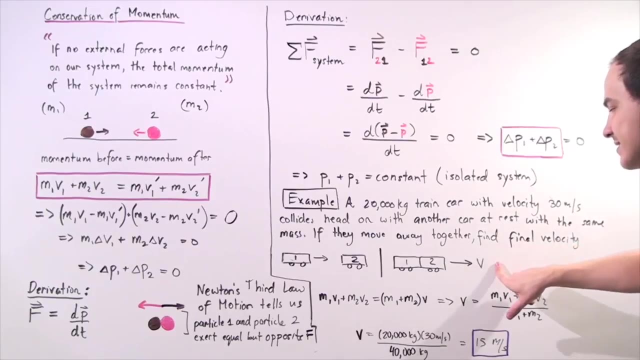 My object 1 is moving in the positive direction along the x-axis with initial velocity of 30 meters per second, and after collision they both move off with the same velocity. So we want to calculate what this velocity is. So we can use this equation where v1. 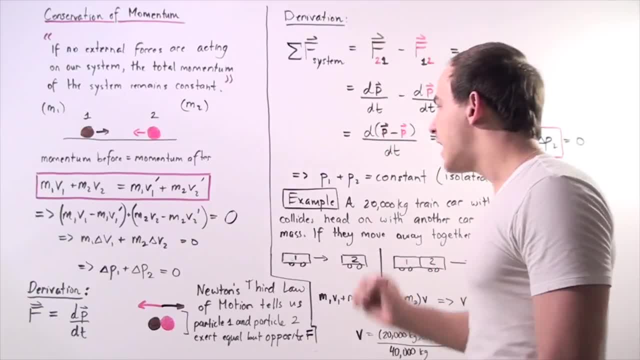 plus the change in momentum of object 2 plus the initial velocity of object 2 plus the initial velocity of object 3 plus the initial velocity of object 3 plus the initial velocity of object 2 and v2 prime and v2- prime are the same exact velocity because they move away together. 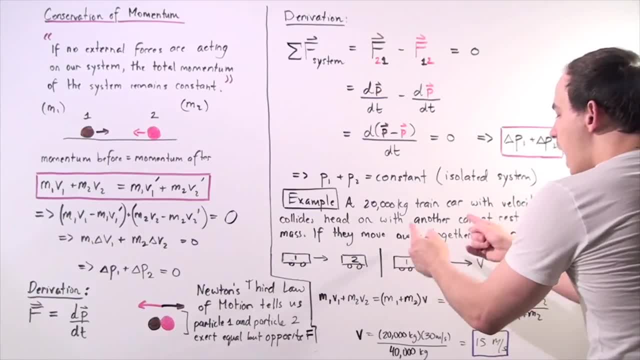 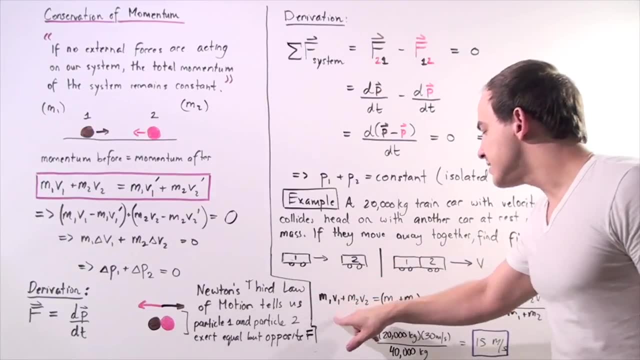 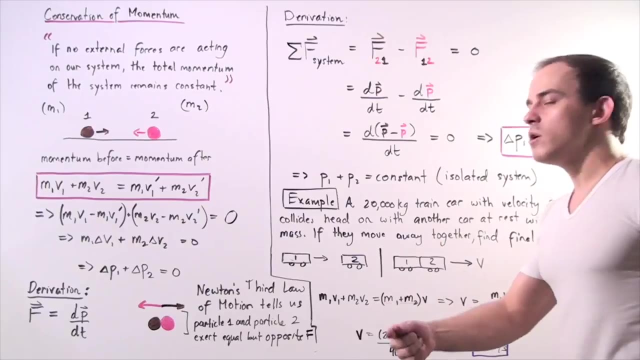 So after they collide it's as if they're one object. So that means we can write the following formula: Mass of object 1 times velocity 1 plus mass of object 2 times velocity 2 is equal to the sum of their masses multiplied by the velocity. So notice, we can solve for velocity. 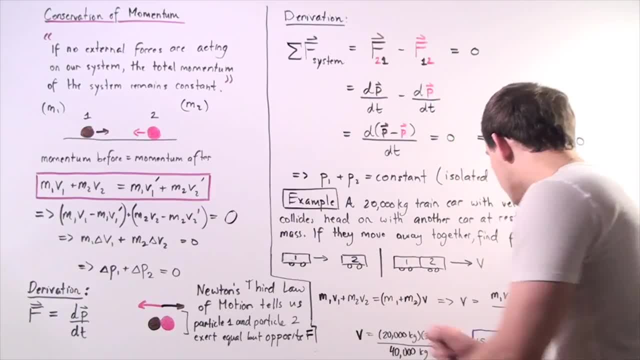 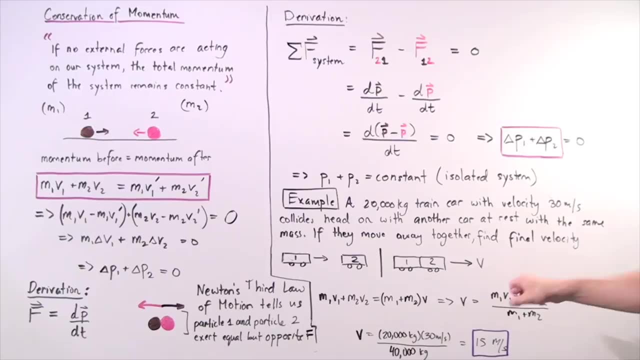 by bringing the mass and the sum of the masses over, and that's exactly what we get. So, because V2 is 0,, we simply have m1 times V1 divided by the sum of their mass, and we get 20,000 kilograms multiplied by 30 meters per second divided by the sum of their masses. 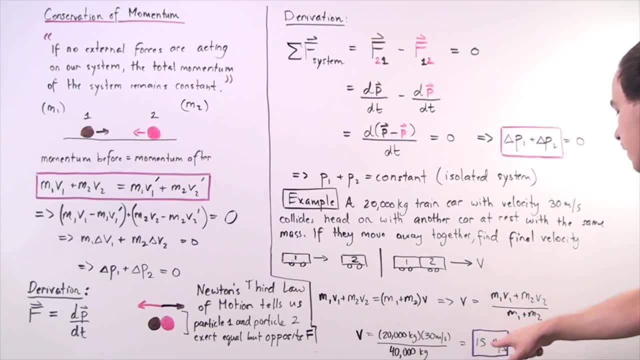 which is twice their mass, is equal to 15 meters per second. So this is the velocity of the objects- both of the objects- after they collide. So we can see how this law can come in very handy.